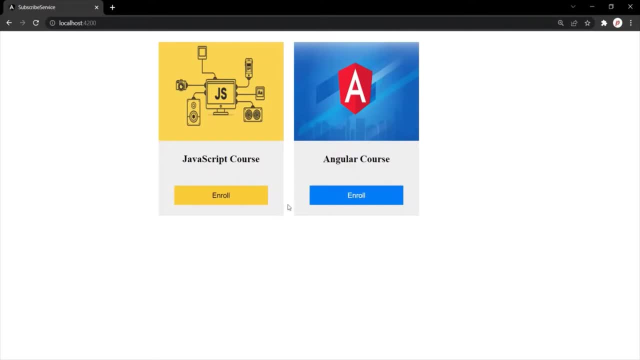 these components has this enroll button. Now, what I want is when a user clicks on the enroll button of JavaScript course, it should show an alert window with the message: thank you for enrolling to JavaScript course, Okay. and when the user clicks on the enroll button of this Angular course. 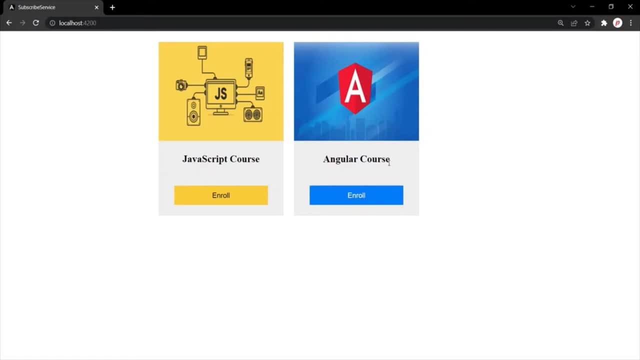 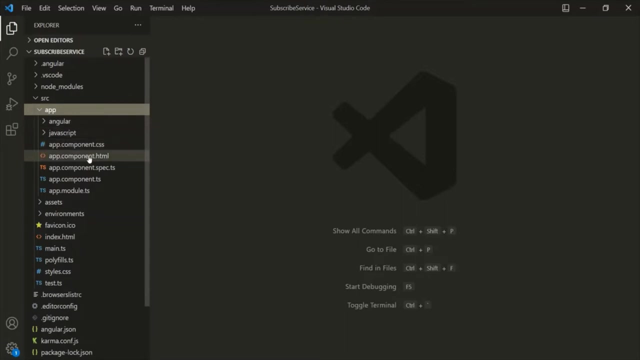 in that case it should disappear. It should display a message: thank you for enrolling to Angular course. Let's see how we can achieve this without using services. So let's go to VS Code. Let's open this source folder, then this app folder, and if I open this app componenthtml, you will notice that here I am using the JavaScript. 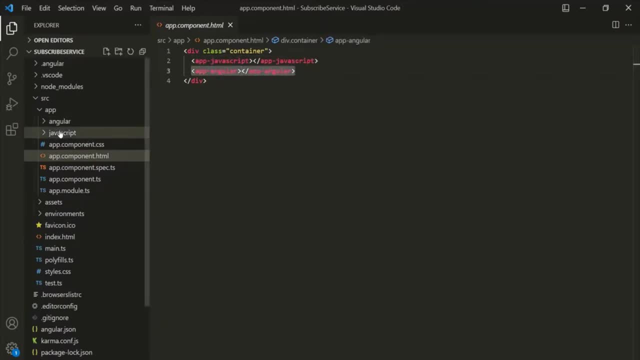 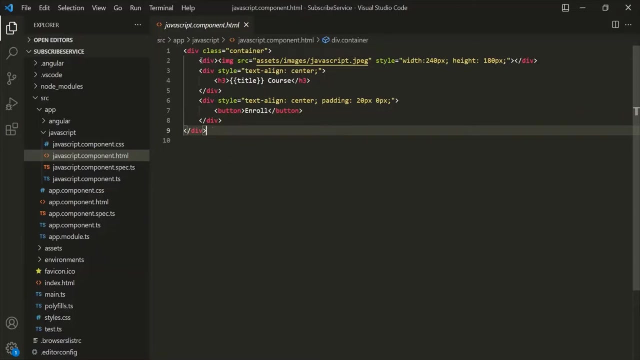 component and the Angular component. So we have these components here. Okay, let's go to JavaScript component first And let's open the HTML file of JavaScript component. Okay, so this is the view for JavaScript component. Inside this view, first we are displaying an image, Then we are displaying the course name. 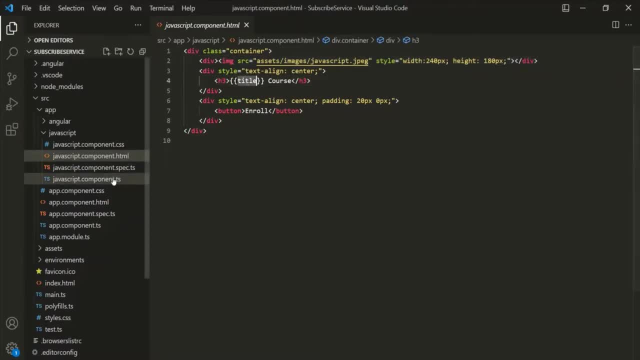 So for that we are using the title property of this JavaScript component. If I go to javascript componentts file here, you will see that this JavaScript component class has this title property, which is set to JavaScript, And we are displaying this value in the view. All right, and then we have: 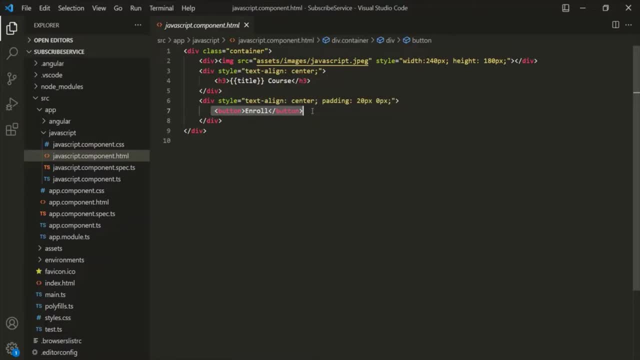 this enroll button. Now what we want? We want that when a user clicks on this enroll button, we want to show an alert message to the user saying that thank you for enrolling to JavaScript course. For that, what we can do is: on this button we can bind click event, Okay, and when this click event happens, 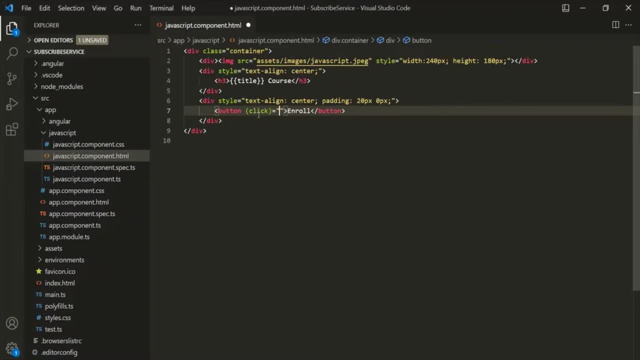 on this button element. let's say we want to execute a method and let's call this method on enroll. Okay, let's go ahead and let's create this method inside the component class of JavaScript component. So let's go to javascript componentts file and inside this JavaScript component class. 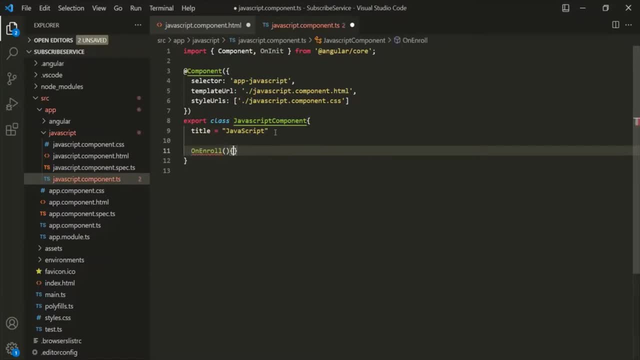 let's define this method, And inside this method, I simply want to call the alert function, And here I want to say thank you for enrolling to, and then let's use the alert function. So let's go ahead and title property. here for that let's say this dot title and then let's also append this string. 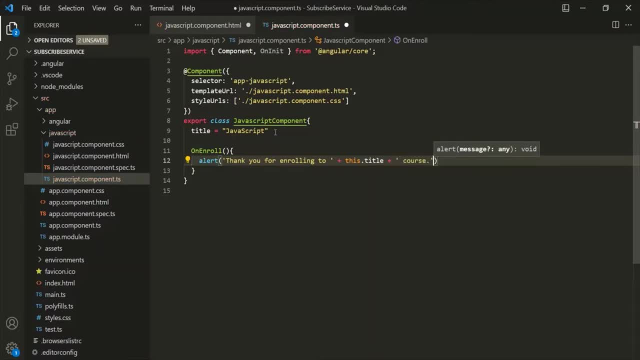 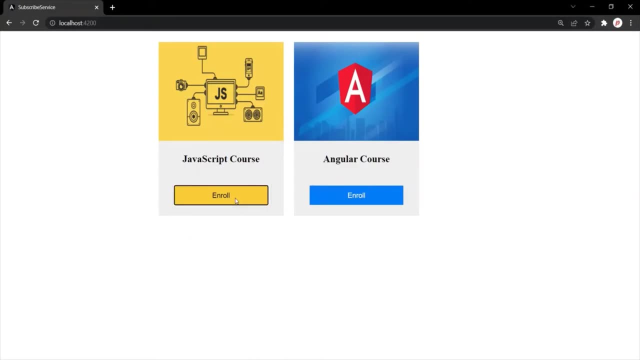 course. okay with this. let's save the changes. let's go to the web page and now, when i click on this enroll button, it should show this alert window with this message: thank you for enrolling to javascript course. okay. now we want to implement the same logic for the enroll button of angular. 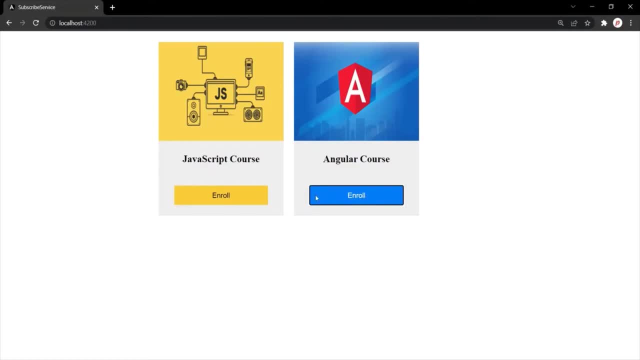 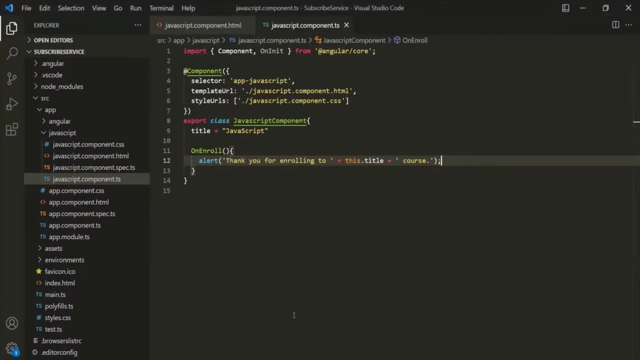 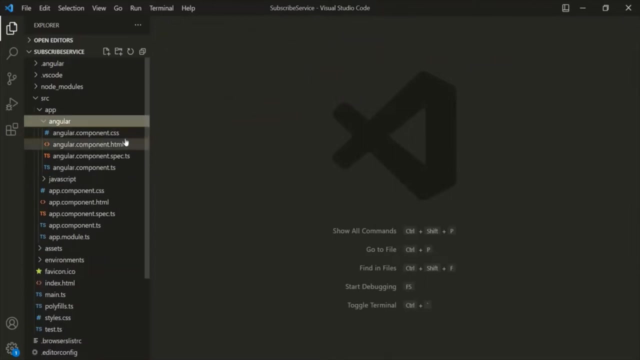 course. so currently, when i'm clicking on this enroll button, nothing is happening. so let's go ahead and let's apply the same logic on the enroll button of angular course. let's go to vs code, let's close this javascript component and now let's open angular component. okay, so let's go to angular. 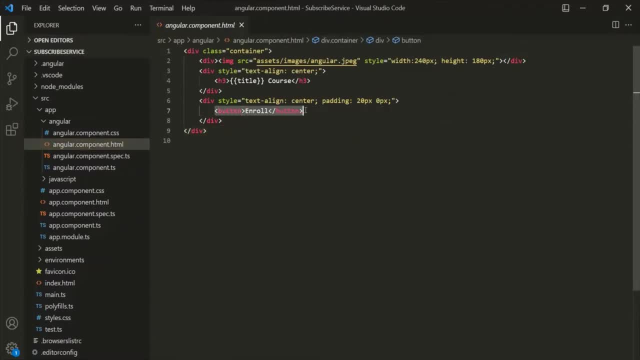 component dot html. and here also we have this enroll button. on this enroll button let's bind this click event and let's call this on you enroll method. okay, and let's go ahead and let's define this method in the component class of angular component. so let's open this angular component dot ts file and let's define this. 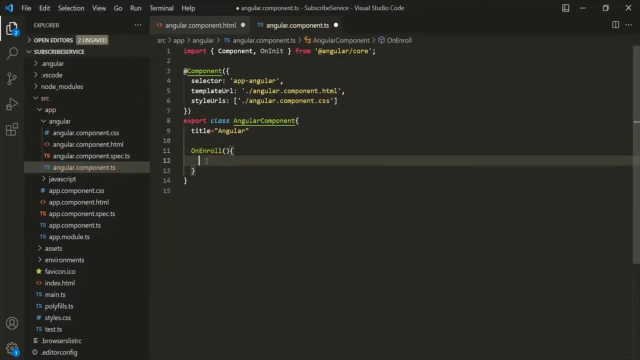 method. here and here we want to display the same message. so let me open javascript component class. so let's open this folder and let's go to javascript component class and from here let's copy this logic: okay, and let's use it inside this. on enroll method. let's save the changes, let's go to the web page. and now, when i click on, 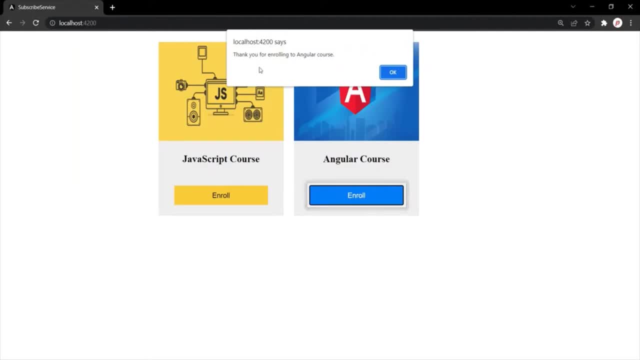 this enroll button of angular course. here also, it should display the alert window with the message thank you for enrolling to angular course, and when i click on the enroll button of javascript course, it is showing thank you for enrolling to javascript course. okay, so this functionality is working as expected. but the problem here is: 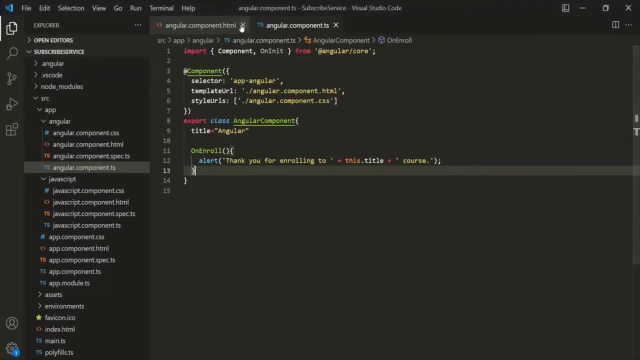 if you notice, if i open this angular component class and if i also open the javascript component class, you will notice that we are writing the same logic in both of these component class. okay, so we have the same method in both of these component class with the same logic. so here we are violating. 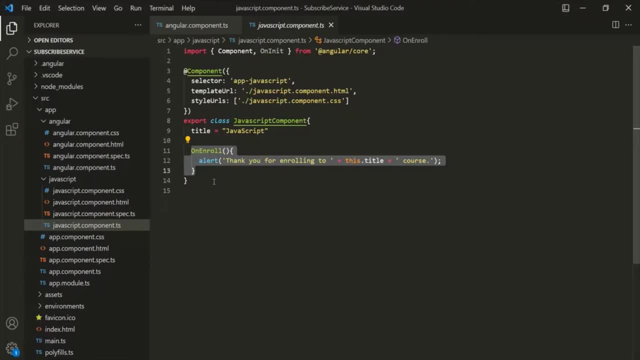 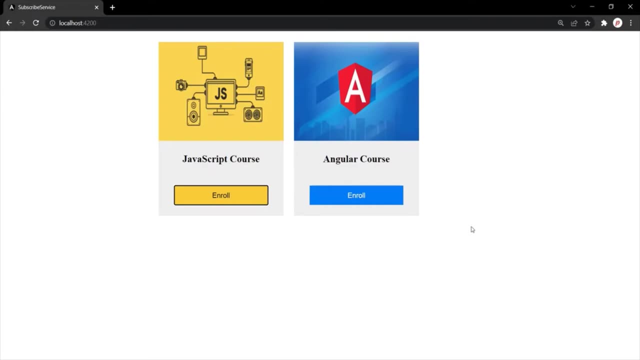 the dry principle: here we are repeating the same code for different components, and if we have more courses in this web page- for example, let's say, if we have a react course and then nodejs course- then for each of those courses in the component class we will have to define this method. 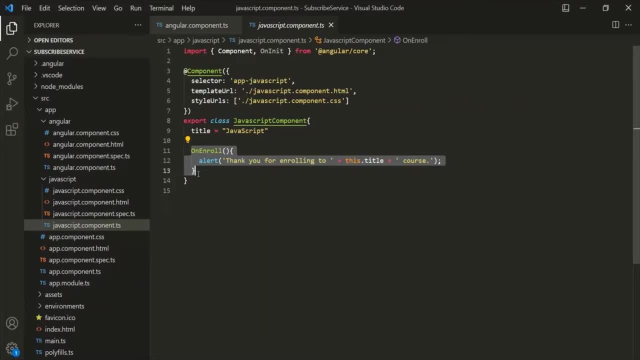 and this is not an efficient way of developing an application. okay, so let's see how we can use services to avoid repeating the same code again and again for different components, and how we can reuse a code. so first let's remove these methods from these components: this javascript component and this angular component. 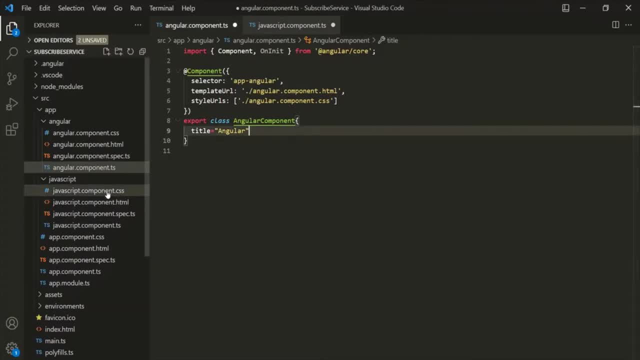 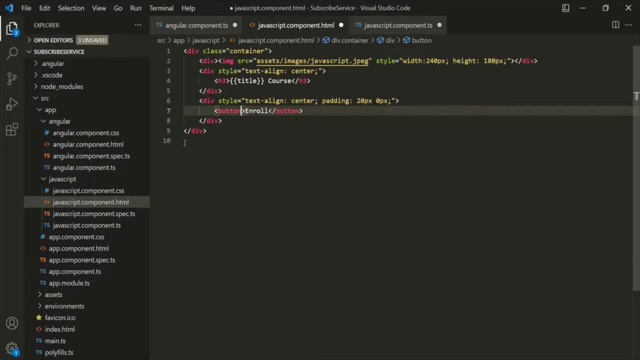 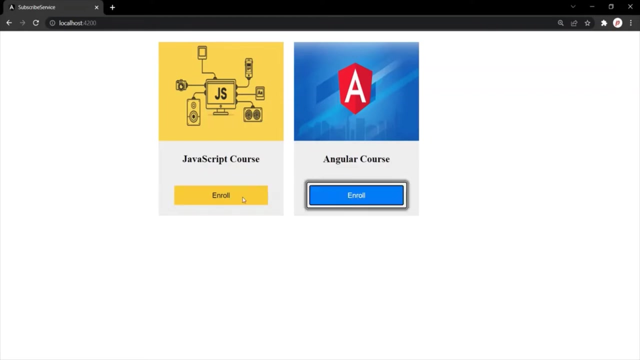 let's also open the html file and, from this button, let's remove this binding of this click event. okay, all right. so now, if i go to the web page, these buttons should not be working now. now let's implement the functionality for this enroll button using services. 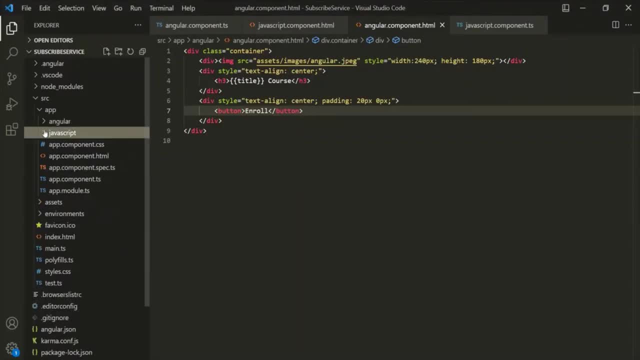 so the first thing which i'm going to do is, inside this app component, i am going to create a new folder and i'm going to call this folder services. so inside this folder we are going to keep all our service files, and inside this folder we are going to keep all our service files. 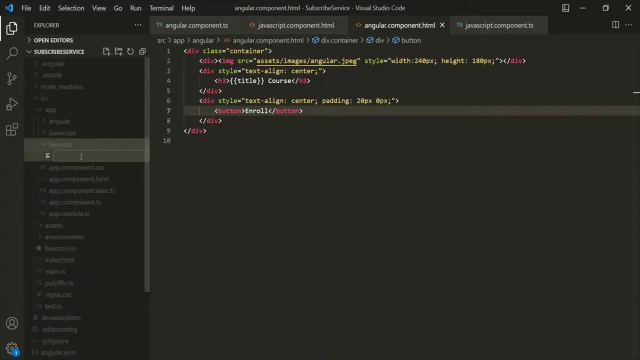 this service folder. let's go ahead and let's create a new file and let's call this file: enroll dot service, dot ts. okay, so this is the naming convention for creating a service file. okay, we use dot service after the service name and it is a typescript file, so we also need to use dot. 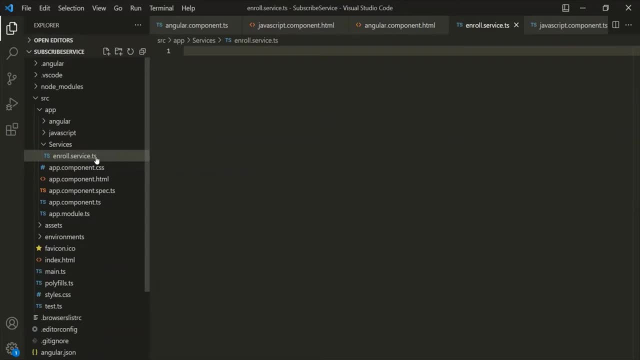 ts extension. all right, so here this enroll service file has been created. now, inside this file, let's create a class and let's call this class enroll service. okay, and let's also export this class. now, when we create a component, we decorate the component class with at component. 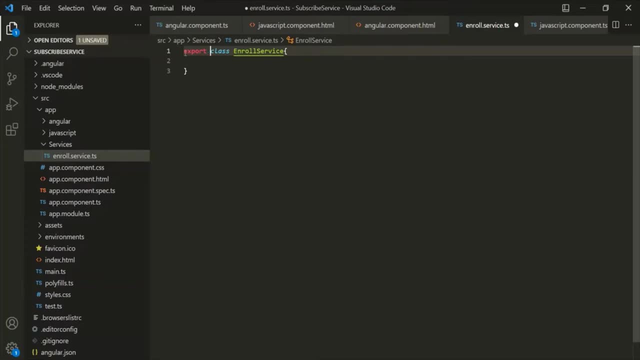 decorator and when we create a directive, we decorate the directive class with a directive decorator. but we don't have to do anything like that in case of a service class. okay, so we need not to decorate this service class with any decorator. a service class is a simple typescript class without any decorator. all right, now, inside this service class, let's 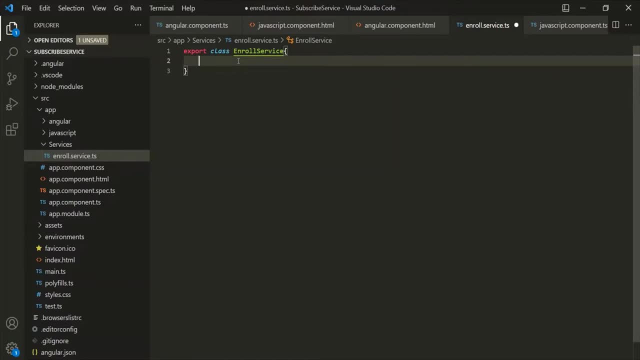 go ahead and let's create a method and let's call this method on enroll clicked, and let's say this method is going to receive a parameter. let's call it title. it is going to be of type string, so this title will be assigned with the value javascript when we will click. 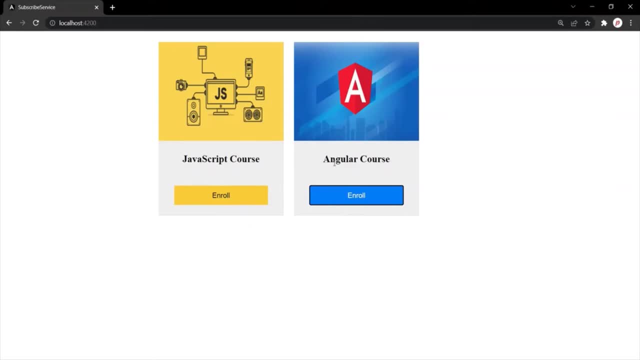 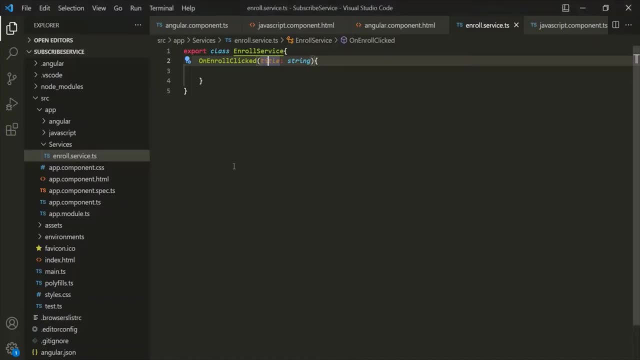 on the enroll button of javascript component and it will be assigned with angular when we click on the enroll button of angular component. okay, and inside this method, let's call the alert function and here let's say thank you for enrolling two, and then let's use the value of the title parameter. 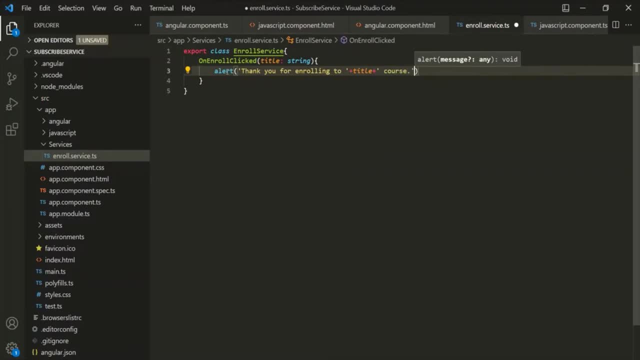 and then let's append this string course: okay, so here we have created this enroll service and this enroll service has this method: on enroll clicked. now what we want is: let me close these files here. so what we want is we want to use this: on enroll clicked inside the angular component. 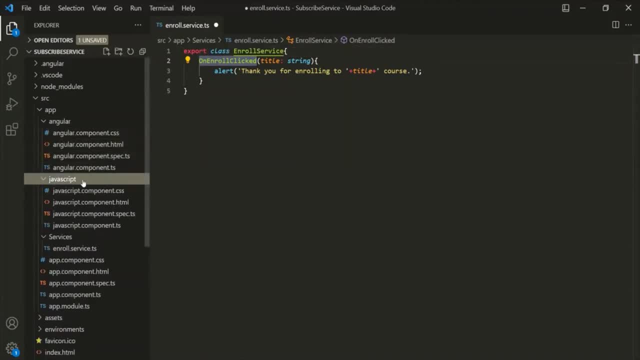 as well as inside the javascript component. okay, so let's go to javascript component first, let's go to the javascript component class and here let's create a method on enroll and from within this method we want to add another function on enroll, want to call this on enroll: clicked method of this enroll service. okay, so for that what we 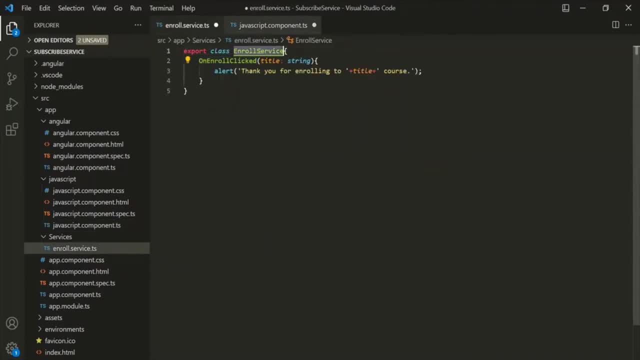 need to do is first we need to create an instance of this enroll service inside this javascript component class. okay, and to create an instance, first we need to create a variable. let's call this variable maybe enroll service, and then to create an instance, we use new keyword followed. 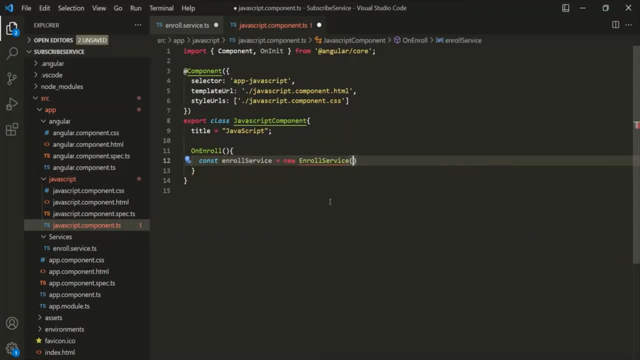 by the name of the class. in this case, the name of the class is enroll service. now, in order to use this class inside this, you know, inside this javascript component file, we also need to import this class from this, you know, from this enroll servicets file. so for that, let's use this. 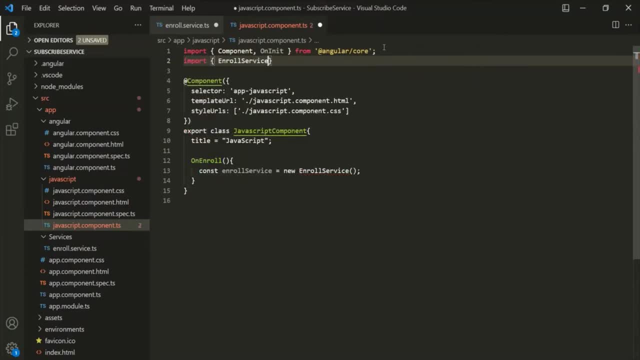 import keyword, and here we want to import this enroll service class from, and then we need to provide the path of this enroll servicets file. so this enroll servicets file is present inside this service folder, right, and we are trying to access it from the javascript folder. 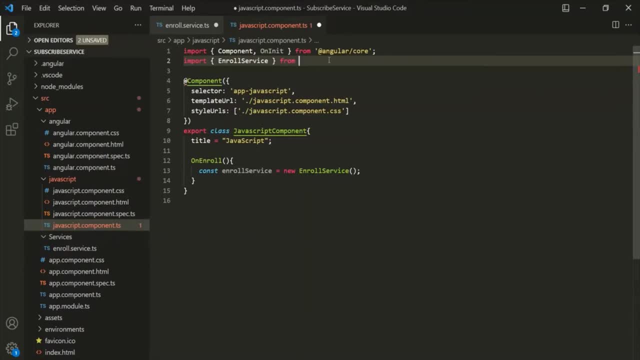 so here what we need to do is first we need to move one folder up to app folder. for that we can use two dots and then a slash. so now we are in app folder, then in this app folder we have this service folder. so here we can say services, and then inside this services folder we have this: 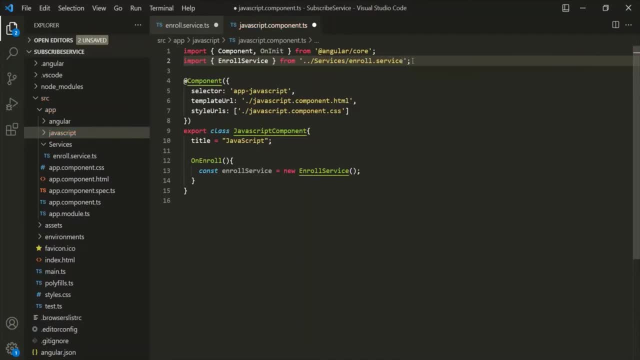 enroll service file. so now you can see we don't have any error here. all right. so once the instance of this enroll service class is created, on this instance we can call that method and the method name is on enroll clicked. and here we also need to pass an argument for this. 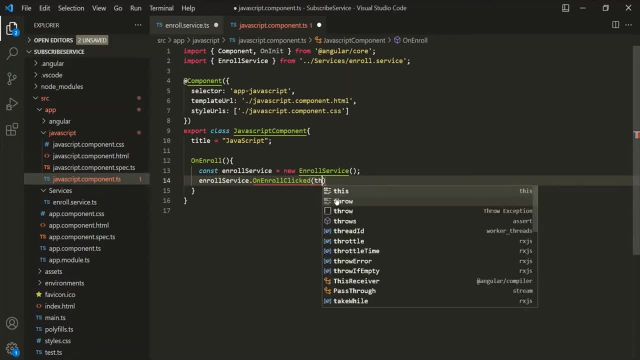 service folder. so here we can say services, and then inside this services folder we have this title parameter. so for that let's pass this dot title. okay, so this javascript component class has this title property and we want to pass the value of that title property to this. on enroll click. 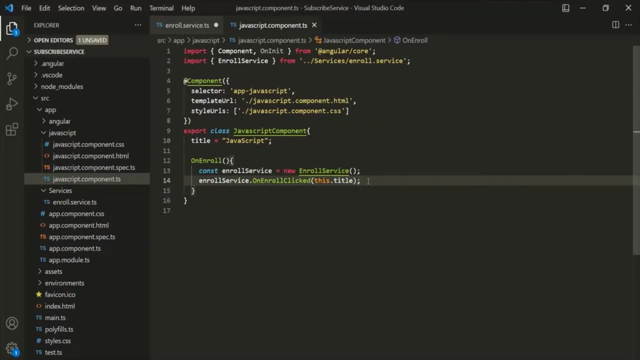 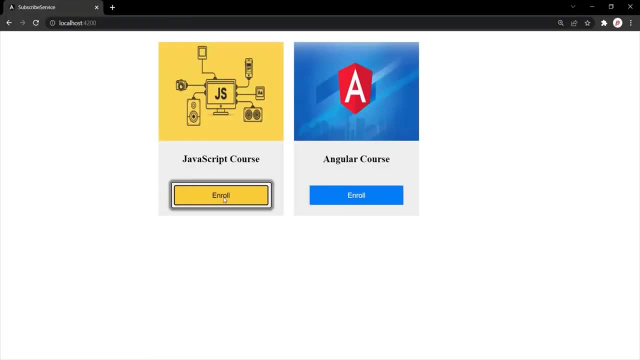 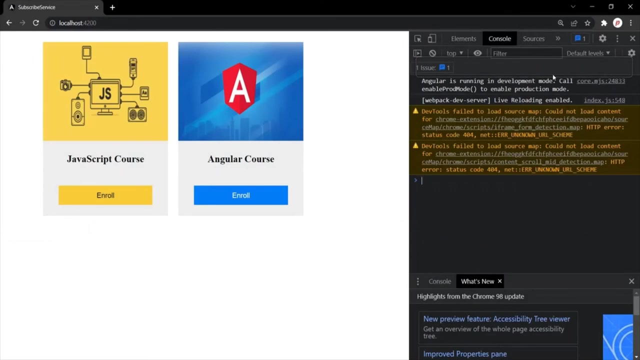 method with this. let's save the changes. let's go to the web page and let me click on this enroll button of javascript course component, and nothing is happening here. let's open developer console so we don't have any error as well. all right now. the problem here is we have created this on enroll method. 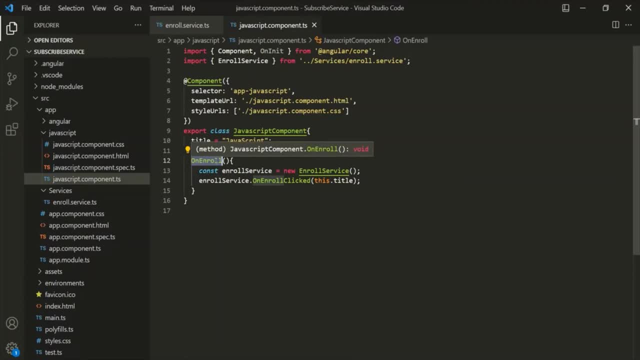 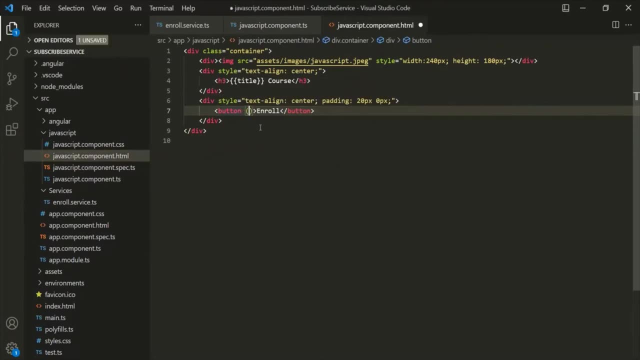 but we also need to bind this method with the click event, right? so let's go to javascript component, dot html file and again on this button let's bind click event and to this click event let's assign this method. so this on enroll method. okay, with this, let's save the changes, let's go to the web page and now this button should be. 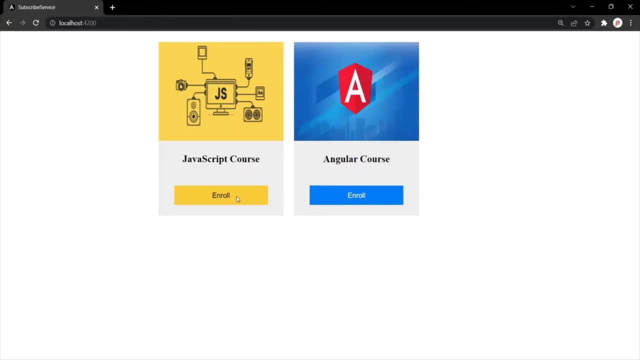 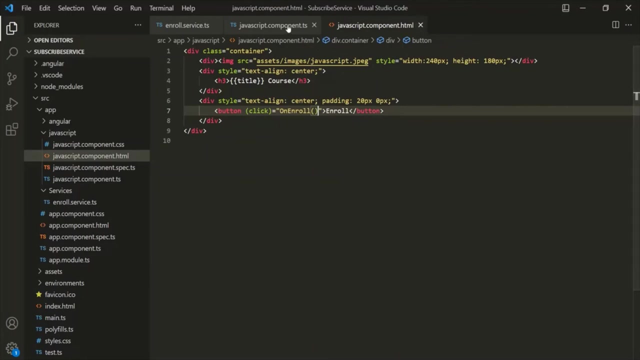 working. so now you can see it is displaying an alert window with the message thank you for enrolling to javascript course. okay, now let's do the same thing for angular component. so let me grab this method from here and let's paste it inside this angular component. let's paste it from: 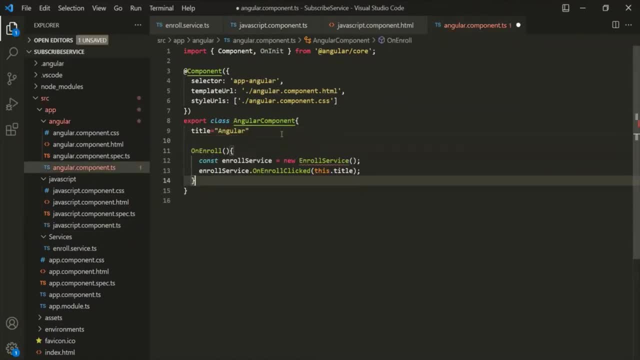 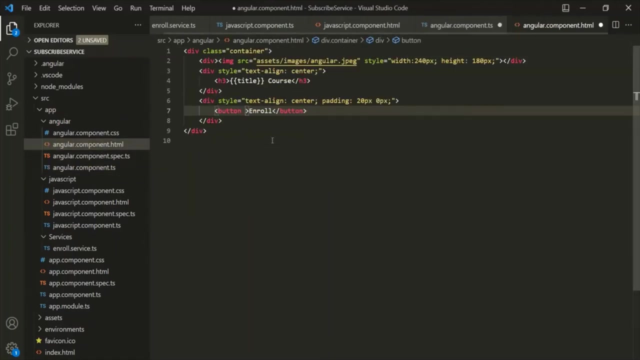 this angular component class. okay, now, in order to use this enroll service class, we also need to import it. so let's get this import statement from this JavaScript component and let's use it inside this angular component. all right, and again, let's open angular component dot HTML file and on the button element: 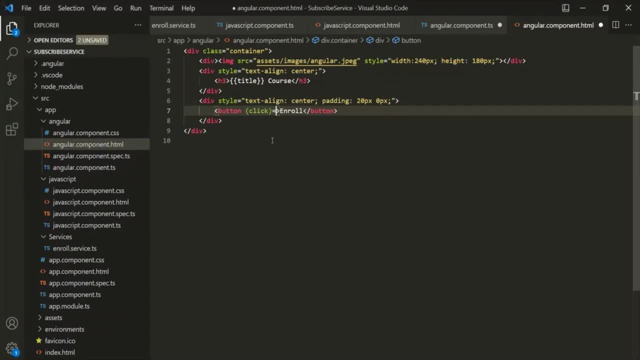 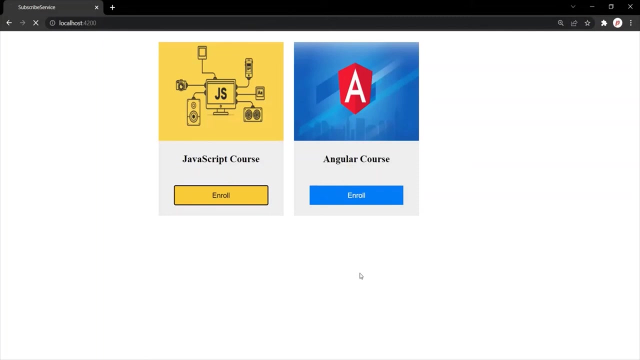 let's bind click event and to this click event let's assign this method, this on enroll method. okay, let's save the changes. let's go to the web page. and now, when I click on the enroll button of this angular component, here also we should get a alert window with the message thank you for enrolling to. 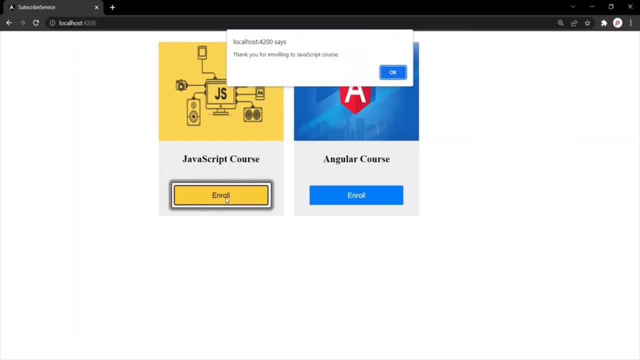 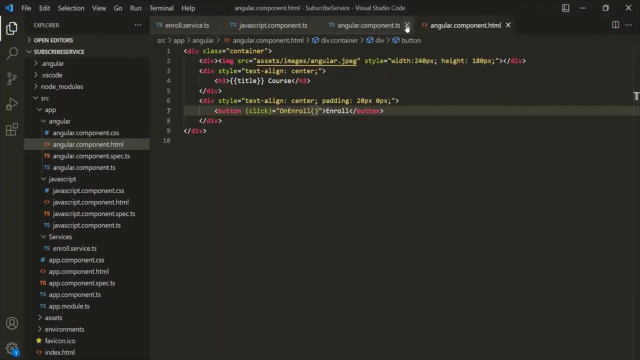 angular course. okay, when I click on the enroll button of JavaScript component, it is showing thank you for enrolling to JavaScript course. so the functionality of this enroll button for both of these components are working as expected. and here we are. let me close these HTML files. so here we are, reusing this on enroll clicked method in the